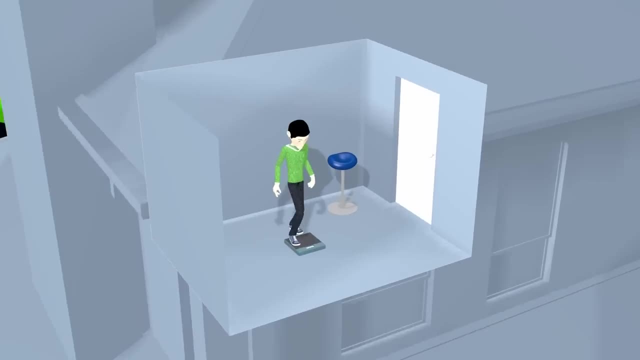 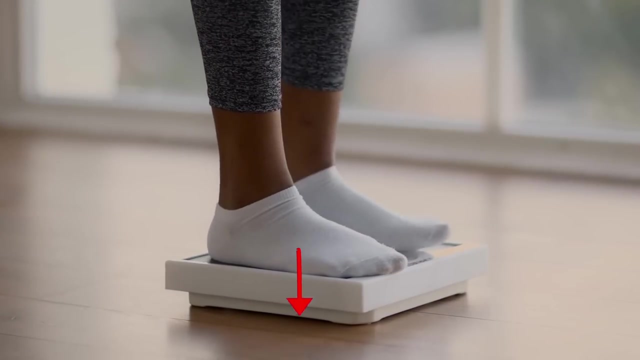 This video is sponsored by Blinkist. When you step on a scale and look down at the number that shows up, what that number is telling you is how much force the mass of your body exerts on the ground. It's simple Newtonian mechanics: Force equals mass, times, acceleration, Gravity exerts. 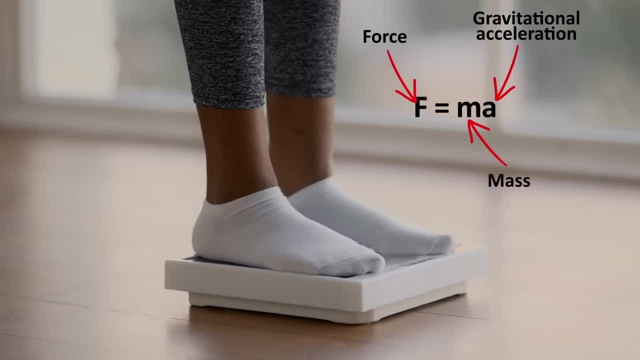 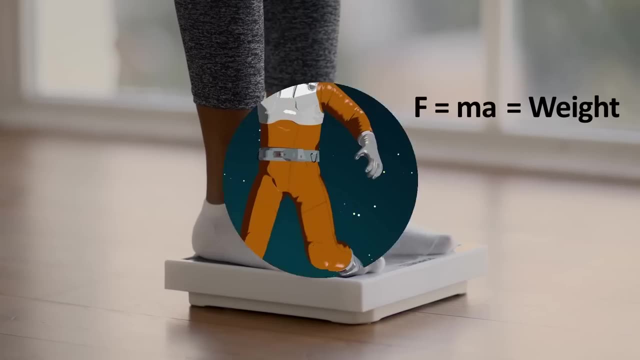 the acceleration on the mass of your body which creates a force That's your weight. So weight is probably easy enough to understand, but mass is a little more nebulous. If you were floating in space far away from earth, you would essentially have no weight, but you would still have the same. 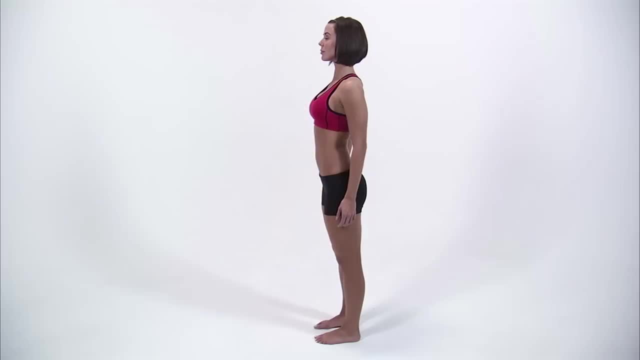 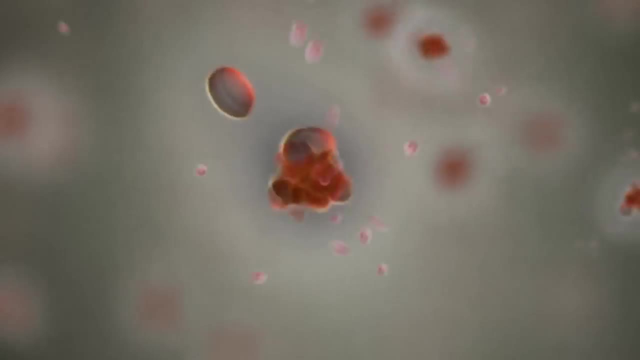 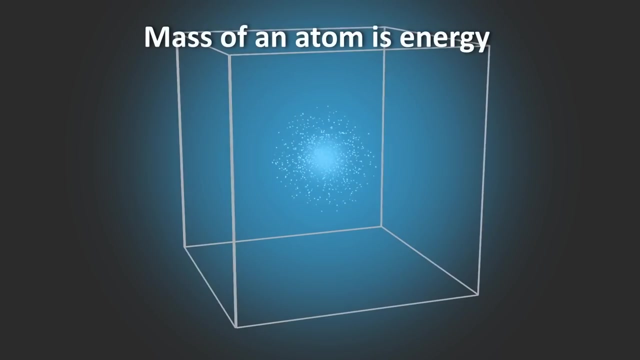 mass, as you did. standing on that scale. Where does the mass of your body come from? Well, the mass comes from all the atoms in your body that individually have a mass. Where does an atom's mass come from? Well, this is interesting because the mass of atoms at its core is really energy. 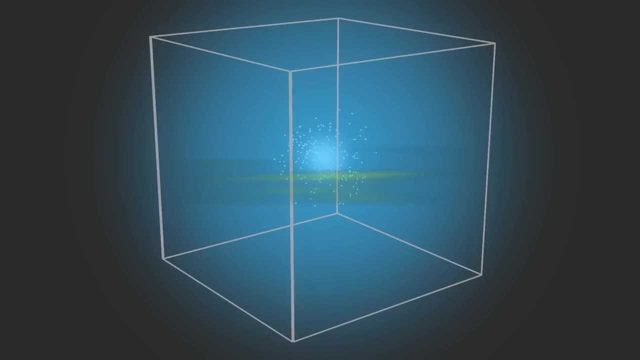 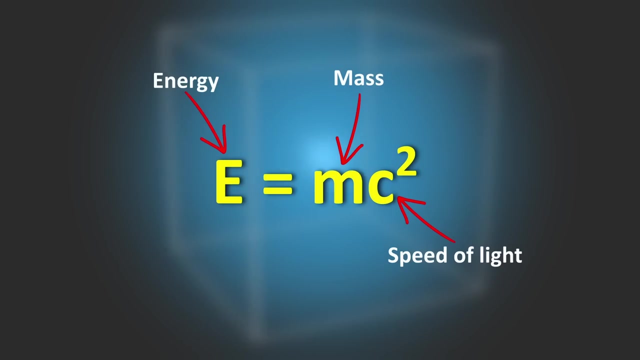 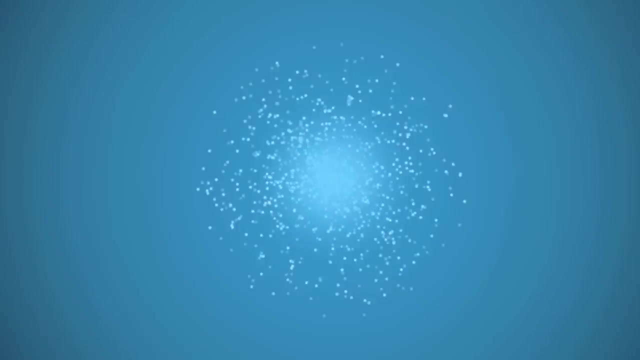 In fact, all mass is energy. This is exemplified in Einstein's famous mass-energy equivalence equation. E equals mc squared. Mass is interchangeable with energy and the constant c squared, or speed of light squared, is the conversion factor. So where is the energy of the atom coming?